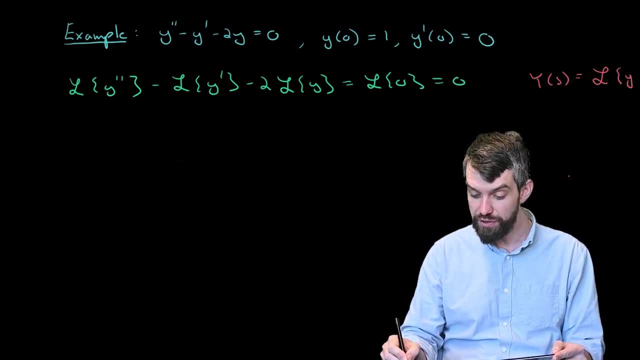 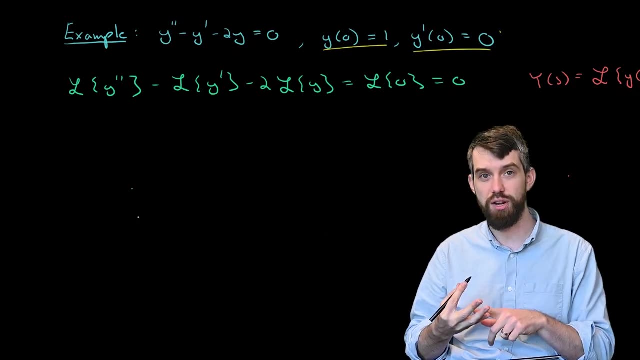 going to be a standing for the Laplace transform of the function y of t that I began with. Okay, so now I need to figure out what is the Laplace transform of the first derivative, the second derivative and so forth. But this is something we computed, actually, in a previous video, So let's do. 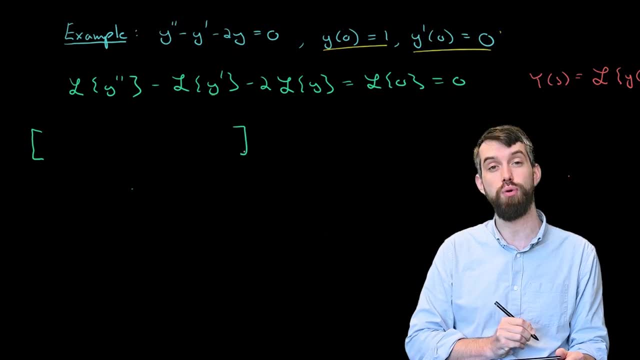 the first one. Let's do the Laplace transform of y double prime. here The expression we had seen was that it was an s squared times y of s, and then it was going to subtract off an s times y of 0, and then subtract off a y prime of 0. That is, it becomes s squared times, this new variable y. 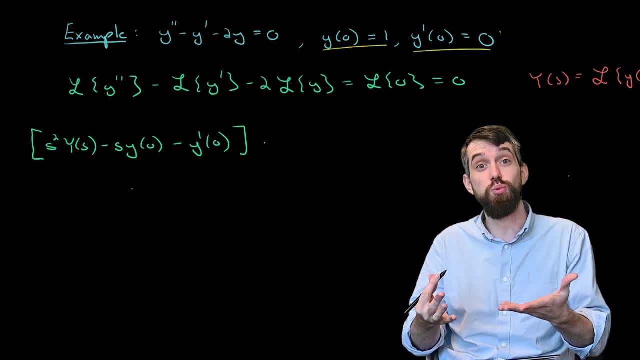 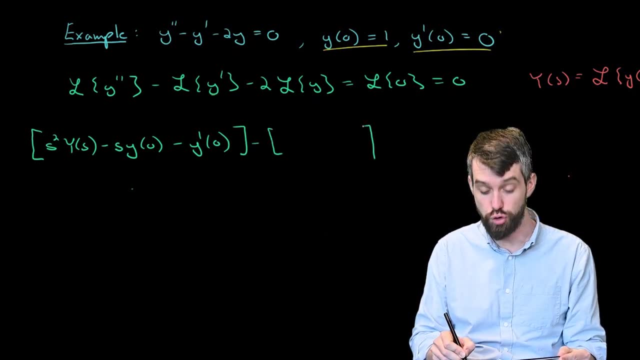 and then it had just two constants: y of 0 and y prime of 0, just constants. We're going to solve that Next up. I need to subtract off the Laplace transform of the derivative. And the first derivative is a little bit simpler, It was s times y of s, and then I suggest: subtract off by y of 0. 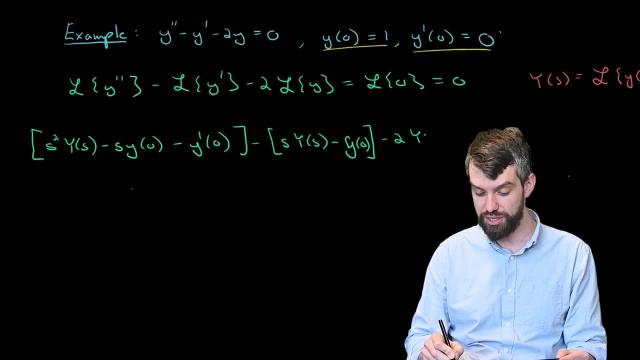 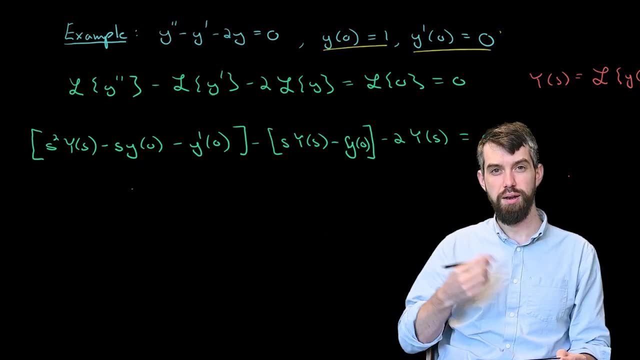 Finally, I subtract off by two times just the Laplace transform of y, which we have defined to be just capital Y of s, and then the right-hand side is once again 0.. Now I'm going to take those initial conditions: the y of 0 equal to 1 and the y prime of 0 equal to 0, and just. 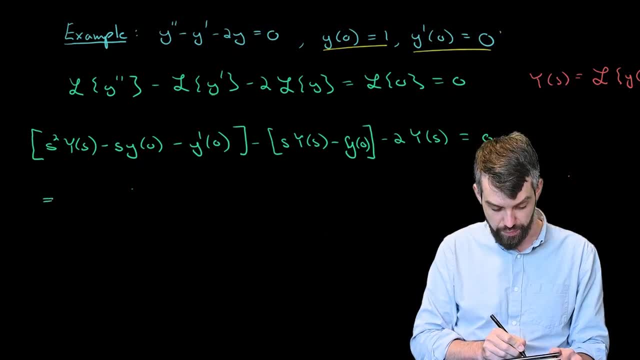 plug them in and let's just see what happens there. This is going to give me well s squared times: y of s. y of 0 was 1, so I'm going to have a subtraction of an s. Then I subtract off just. 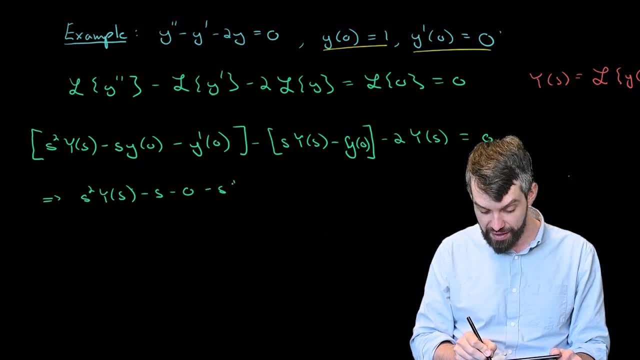 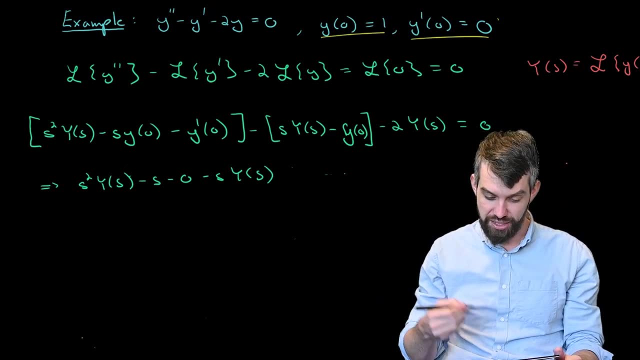 nothing, so minus a 0.. Then I subtract off s times y of s. I then have another subtract off y of 0, but it's got two minus signs now and, as a result, it's going to give me a plus 1,. 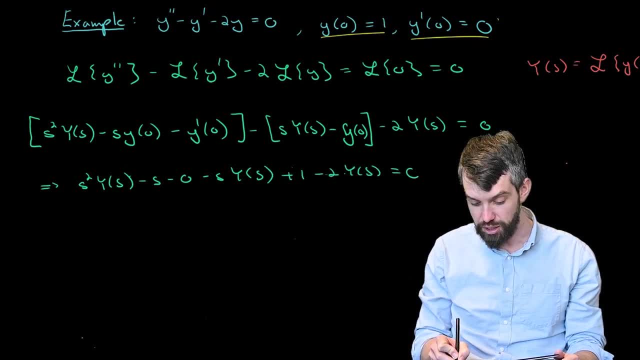 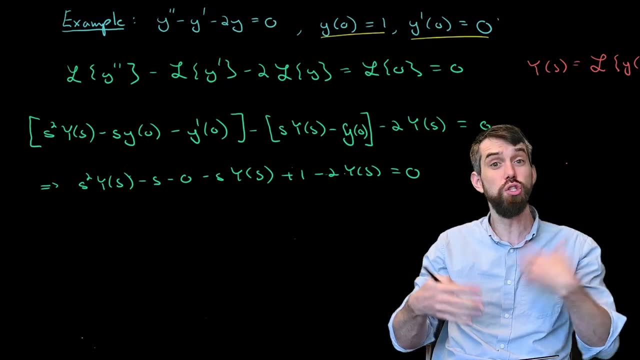 and then a minus 2 times y of s, and all of this is equal to 0.. Now, this is a little bit complicated, but I'm going to show you how to do it. I'm going to show you. the equation that I have here is an equation in terms of the variables y and s, and I want to solve. 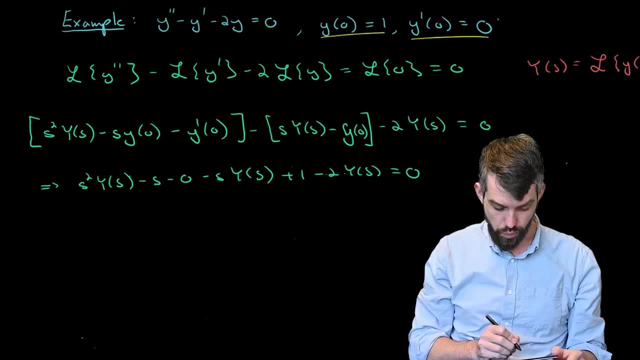 it so that y can be written as some function of s. The way I do this is I'm going to try to make y of s be on the left-hand side. so what's on the right-hand side? Well, everything else looks like. 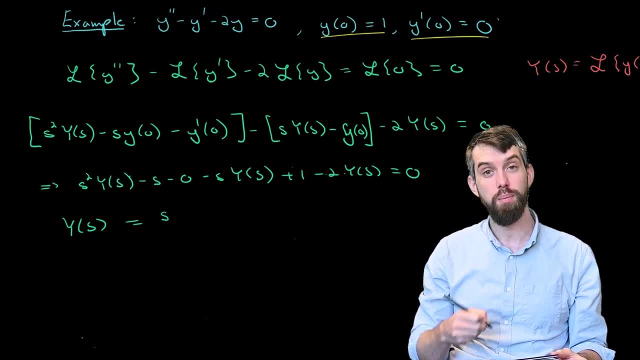 a minus s that's going to move over and become a plus s, and then a plus 1 that's going to move over and become a minus 1.. And then I'm going to divide out by the coefficients of y of s, which looks like an s squared, a minus s and a minus 2.. 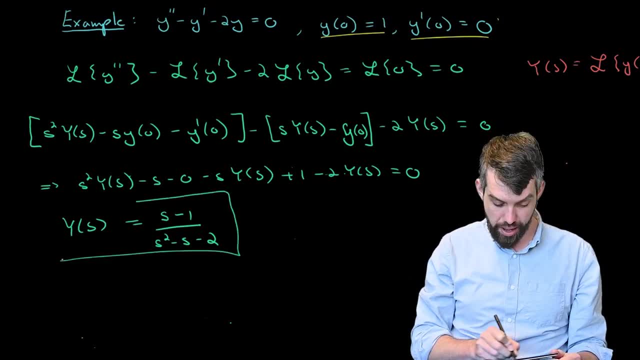 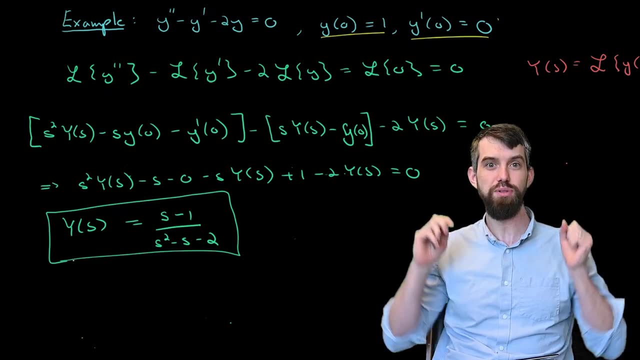 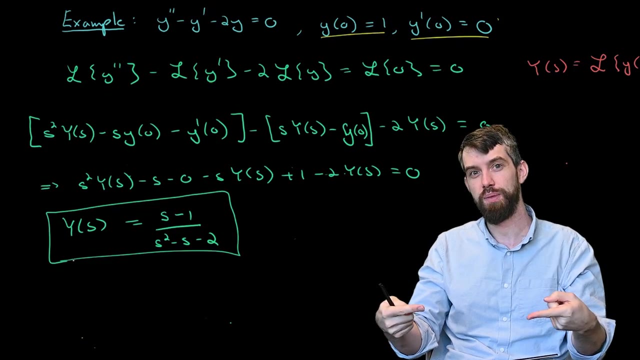 And so that is my answer, That is, algebraically solving for y as a function of s. Now I'm not done yet. I took this differential equation and I converted it via the Laplace transform to an algebraic equation and I solved that algebraic equation, But I don't yet have a solution to the. 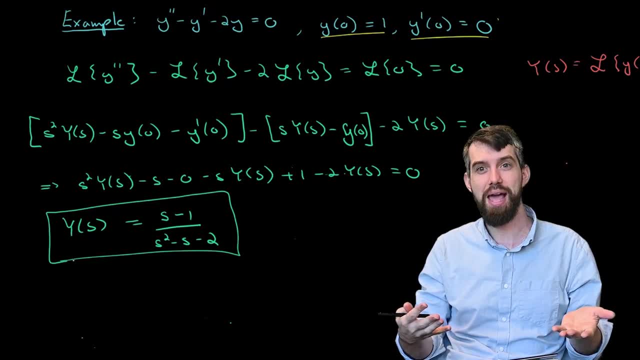 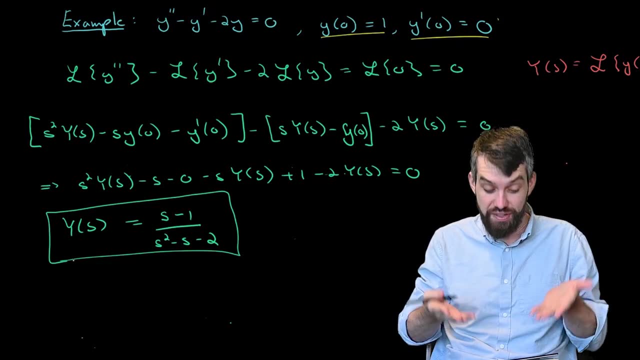 original differential equation. so I have to undo the process somehow. I have to apply the inverse Laplace transform. So the question is: what is the inverse Laplace transform of this thing, of this s minus 1 over s squared minus s minus 2?? So that's what we're going to turn to next. 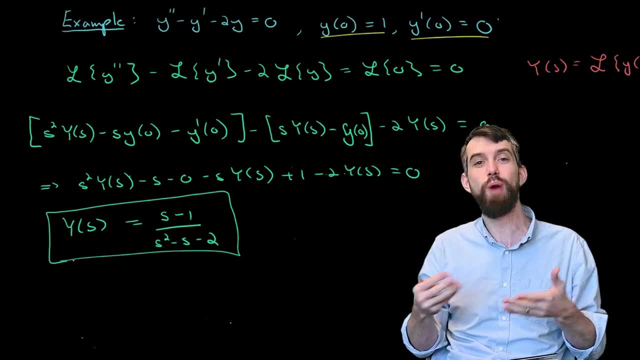 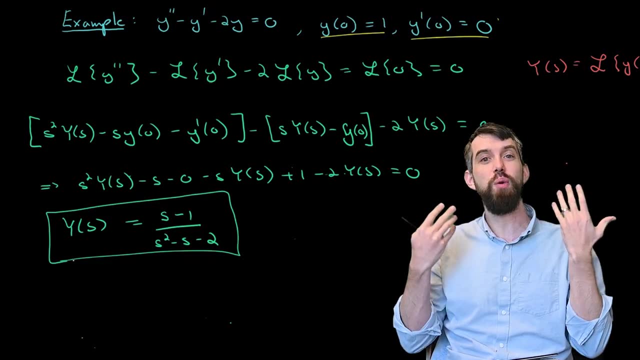 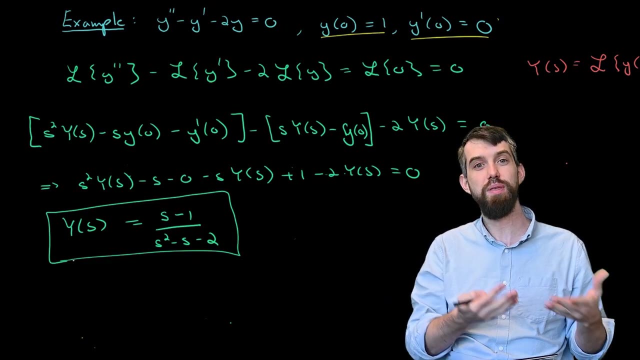 And the way we do this in general is to try to recognize these functions that we want to take the inverse Laplace transform of, try to recognize them in terms of things that we already know, in terms of expressions that we already know, their inverse Laplace transform of, And the major. 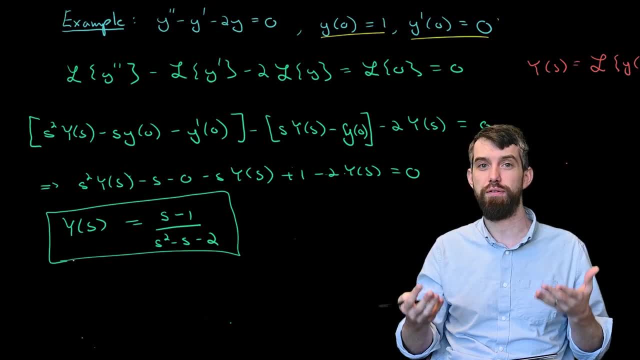 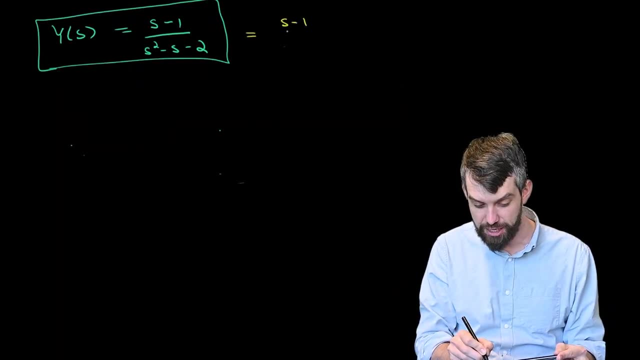 algebraic trick I'm going to use to do that is partial fractions. So let me recall how that works. All right, so my first trick is just going to be to factor, and I see that in the denominator I can write this as s minus 2 times s plus 1.. Then the magic of partial fractions is that. 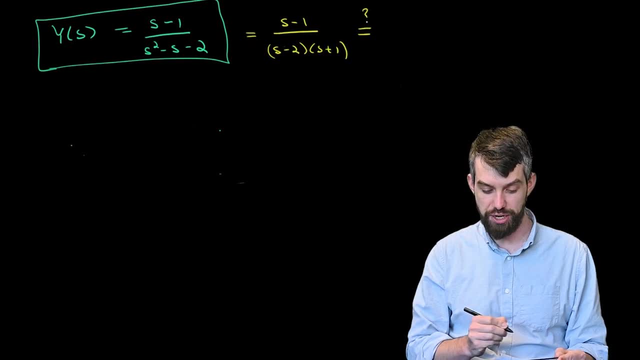 we aim to write this complicated rational expression as a single variable: a over the first linear factor, which is s minus 2, and then a second b over the second linear factor, which is s plus 1.. And then the way partial fractions work. 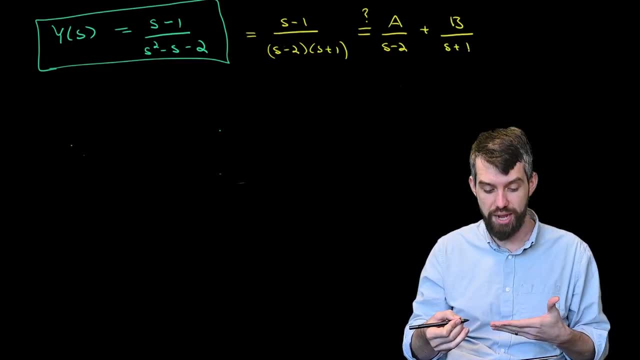 was: let's multiply both sides by the denominator. here this s minus 2 times s plus 1.. And that's going to give me that on the left-hand side, when I multiply it by the denominator, I get s minus 1.. 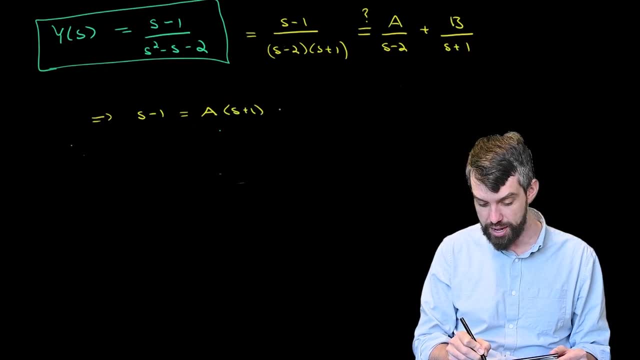 And on the right-hand side, a times s plus 1 and b times s minus 2.. There's several ways to proceed here, but the way I'm going to look at it is- I'm going to do the coefficients of the 1.. On the left-hand: 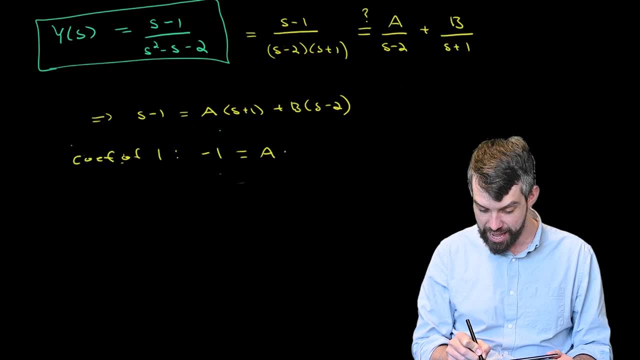 side, the coefficient of 1 looks like an a and then a minus 2 b. Likewise, I'm going to compute the coefficients of s, which on the right-hand side looks like there's one s And on the right-hand side there's an a times an s and a b times an s. So what I've done here, by looking at the 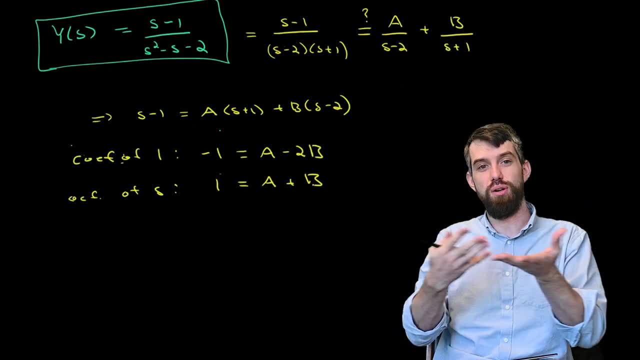 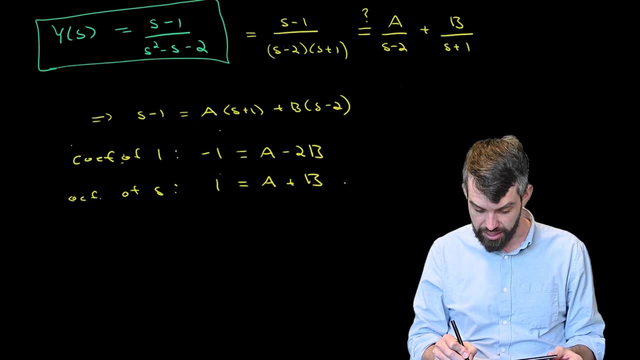 coefficients of 1 and the coefficients of s is to take this single equation and actually think of it as two separate equations, one in s and one in terms of 1.. Well, we can solve these easily enough. If I look at the bottom expression, that's going to give you that a is 1 minus b. 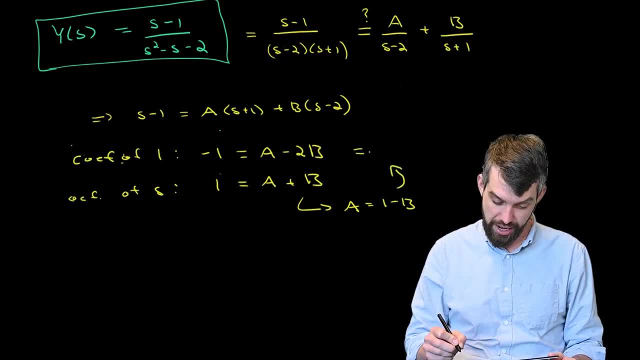 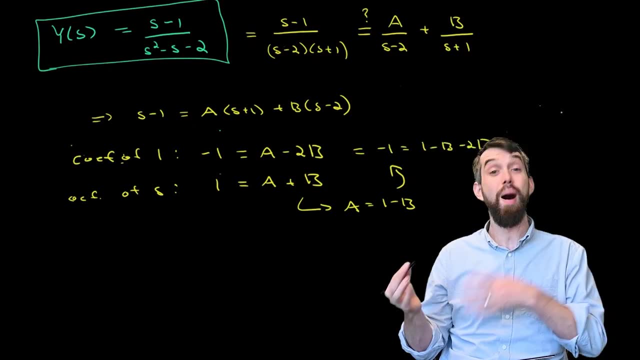 And if I take that and plug it into the top expression, then this is going to give me that minus 1 is equal to 1 minus b minus 2b. So I have a minus 2 on the left If I move the 1 over. 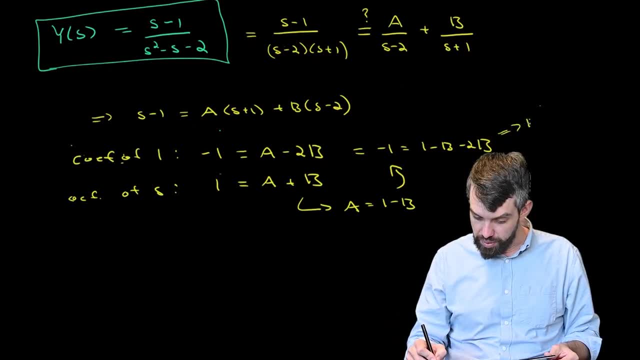 a minus 3. And so my b is 2 thirds. So b is 2 thirds, And if the a is 1 minus 2 thirds, then that's going to imply that the a is equal to 1.. So I figured out what my a is and I figured out what my b is. 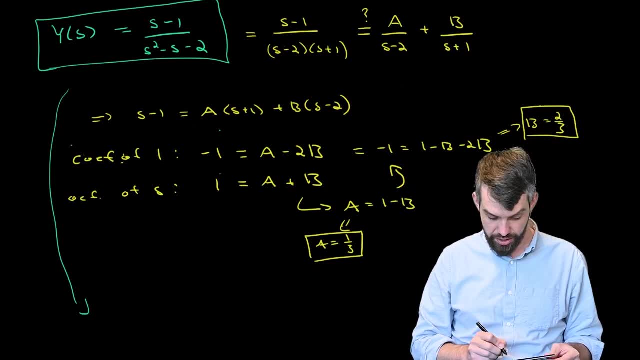 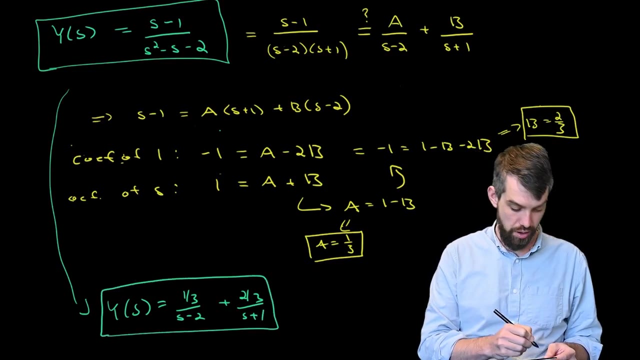 All right. So, having done that partial fraction stuff, I'm going to come down here and take this expression of y of s And I am now going to write it as 1 third over s minus 2 and 2 thirds over s plus 1.. This is my rewriting of this expression. OK, So let's move that up as well. And then we 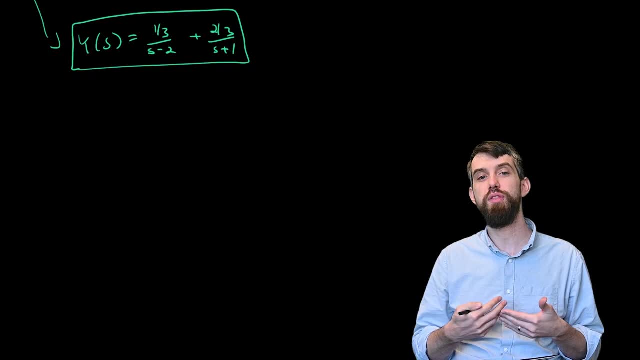 can study it. Well, my final goal was is to compute the first Laplace transform of this, But now I've finally written it in a way that I can understand, And the reason is because I know a Laplace transform that looks like this In particular: 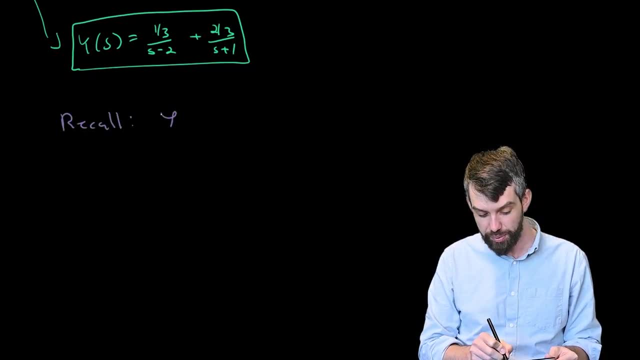 I will recall for you the fact that the Laplace transform of something of the form e to the at this was nothing but 1 over s minus a, And indeed this y of s just looks like 1 over s minus a for two different values of a: 1 being minus 2 and 1 being minus 2.. And so I'm going to take that.